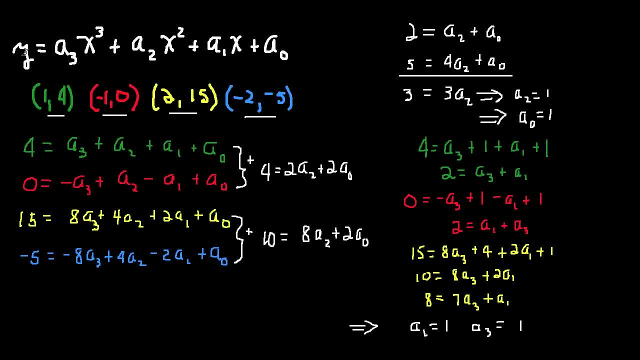 So I plug in x equal 1 and y equal 4 into this equation for the polynomial. So y equal 4 is equal to a cubed times 1, cubed, which is 1, plus a2 times 1 squared, which is 1, so we get a2, plus a1 times 1, which is a1 plus a0.. So the first point here gives us this equation that must be satisfied by the coefficients a1 and a2.. 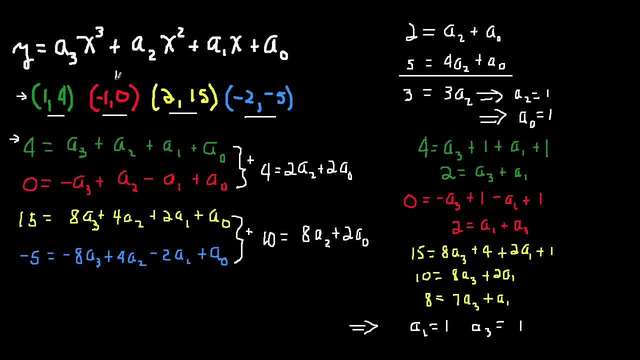 a0 through a3. Now let's plug in the red point right in here And then we write down the red equation: x is equal to negative 1, y equals 0. So we get y equals 0, equal to a3 times negative 1 cubed, That's a negative a3.. a2 times negative 1 squared. negative 1 squared is 1.. So that's a2 plus a2.. And plus a1 times negative 1, which is minus a1.. 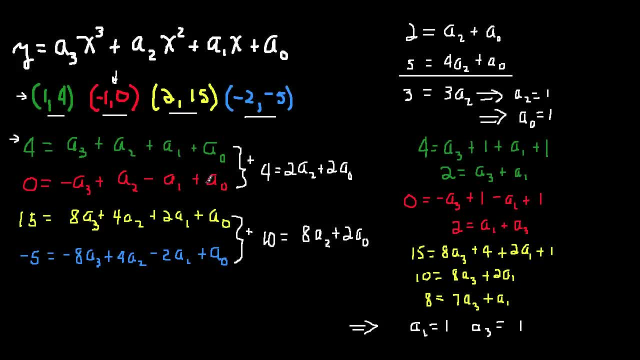 And then plus a0.. a0, bring that down. So the red point gives us this equation that must be satisfied by the coefficients a0 through a3.. Let's look at the yellow point: y equal 15,, x equal 2.. So we get 15 equal to a3 times 2 cubed. 2 cubed is 8, so that gives us 8a3. 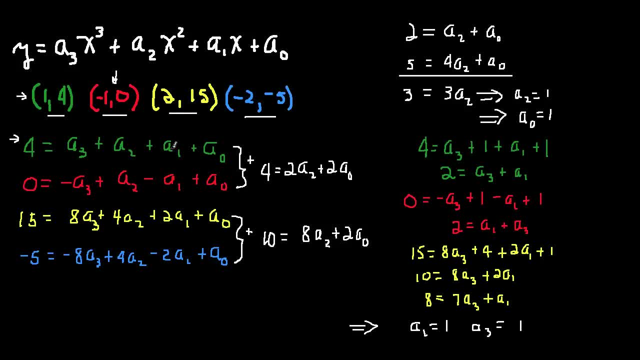 We get a2 times 2 squared, That gives us 4a2.. We get a1 times 2.. That's 2a1 plus a0.. So the yellow point says these four coefficients must satisfy this equation. And then finally the blue point here negative 2,, negative 5, gives us this equation if you plug it in. 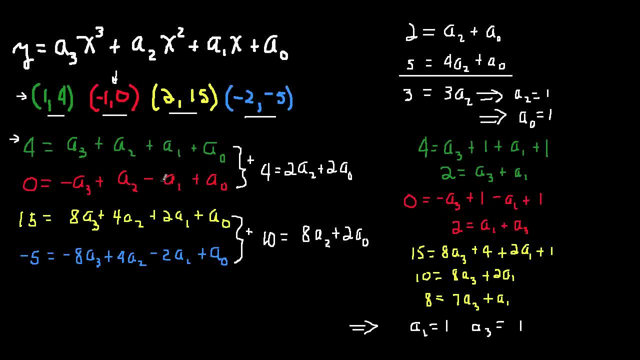 Okay, So we have four equations, all of which must be satisfied by the constants a0 through a3. That are the coefficients in our cubic polynomial. Okay, so I need to solve these four equations for a0, a1,, a2, and a3. 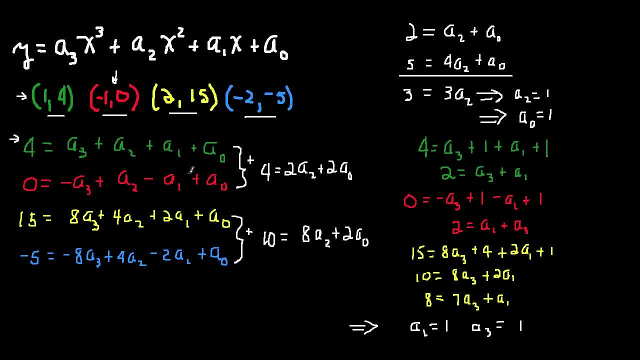 So I'm going to begin that process by taking the green equation and the red equation and simply adding them together. So I'm going to add these two equations together: 4 plus 0 gives me 4.. An a3 and a minus a3. 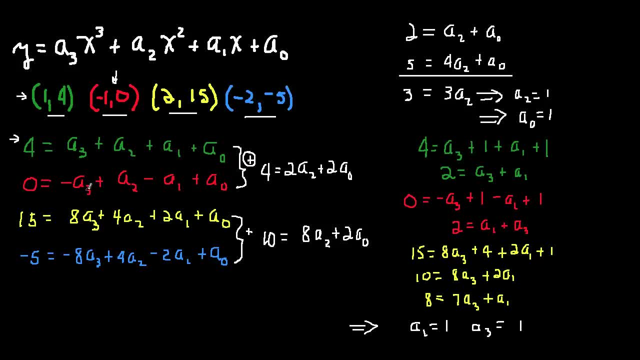 A negative a3 added together gives me no a3.. A2 plus a2 is 2a2, so that's this term right here. A1 minus a1, that gives me 0, a1.. And then a0 plus a0 gives me 2a0. 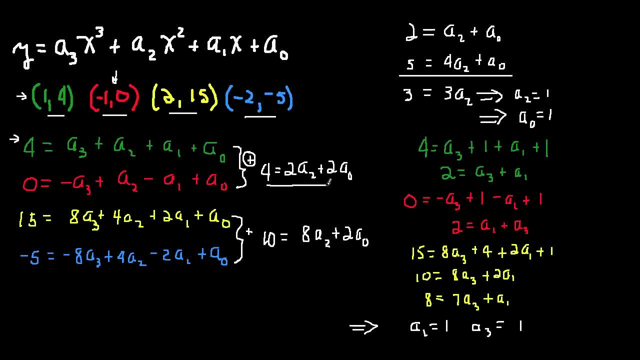 So adding these two equations together gives me this equation: right here Must be satisfied by a0 and a2.. Now let me add these two equations together. I add them together: 15.. Minus 5 is 10.. 8 a3 minus 8 a3 is 0.. 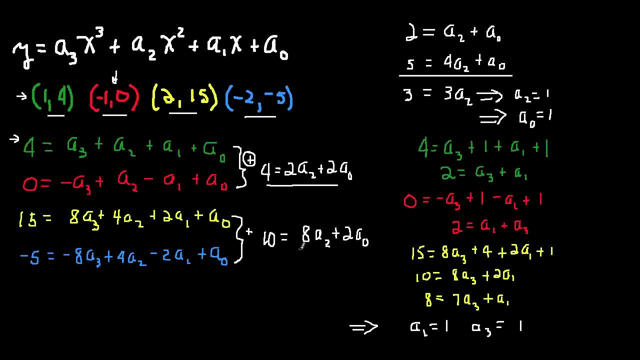 4 a2 plus 4 a2 is 8 a2.. 2 a1 minus 2 a1.. This is an a1 here. in case it's not clear, This is 0.. And then a0 plus a0 gives me 2a0. 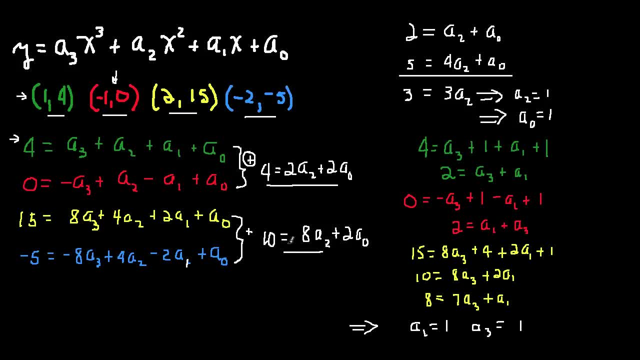 So I add these two equations together Gives me this result. So now we have these two expressions which I have now copied up here, Except With this equation right here. I've divided it by 2 on both sides. It gives me 2 is equal to a2 plus a0. 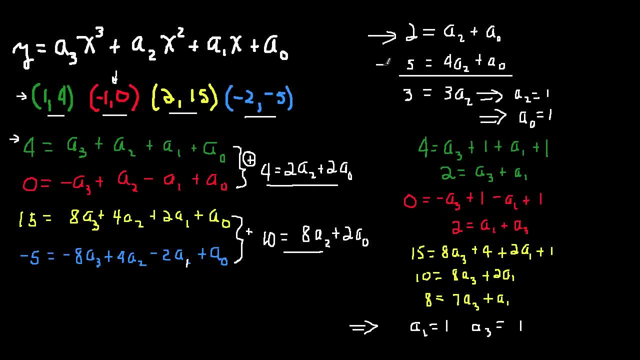 This equation I've divided by 2. It gives me 5 is equal to 4a2 plus a0.. So now I have these two equations directly from these two. So these two up here give me these two equations up there. Okay, now I take these two equations. 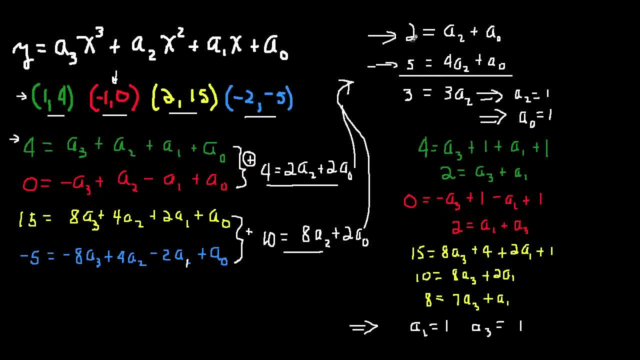 And I'm going to subtract the top one from the bottom one: 2 from 5 gives me 3.. a2 subtracted from 4a2 gives me 3a2.. And a0 from a0 gives me 0.. 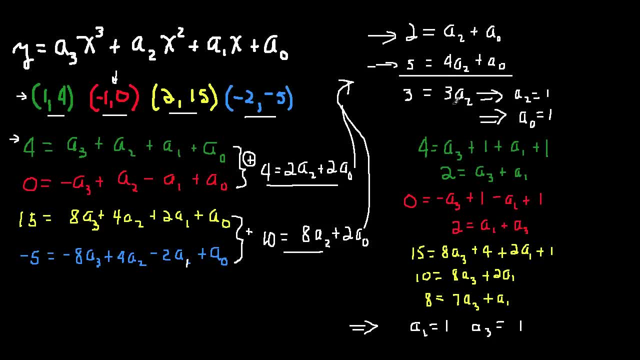 So I get 3 equal to 3a2.. And which is pretty straightforward, Gives me that a2 must equal 1.. Well, if a2 is equal to 1, I can go back and put 1 in this equation for a2.. 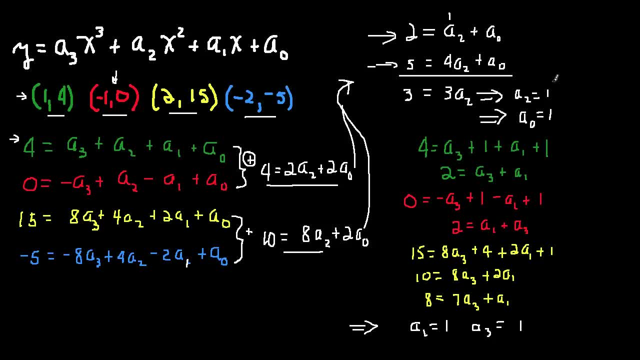 And I see that a0 must also equal 1.. So I get these two equations or these two values for a0 and a2.. Okay, now let me now see With these two values for a0 and a2, can I go back plugging? 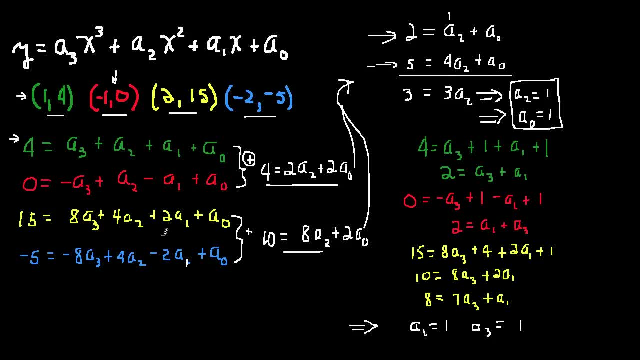 into these equations to give me a1 and a3?. Well, if I plug into a, into the first equation, Because I've got a1.. Because that's the simplest one, I have 4a3 plus a2, which is 1, plus a1 plus a0, which is 1.. 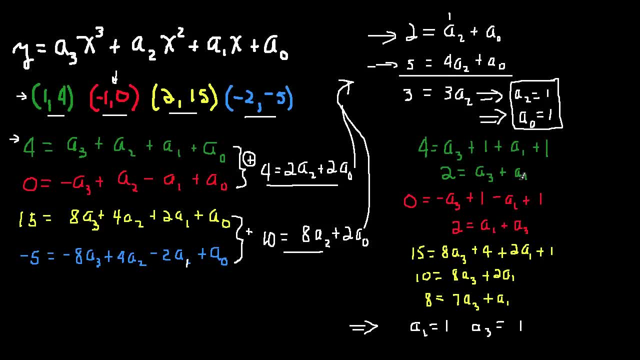 And that gives me 2 equal to a3 plus a1.. Okay, Now, if I plug into the red equation, I get 0 equal to negative a3 plus a2 plus a2 here, which is 1.. And then I get 2 equal to negative a3 plus a1 minus a1. 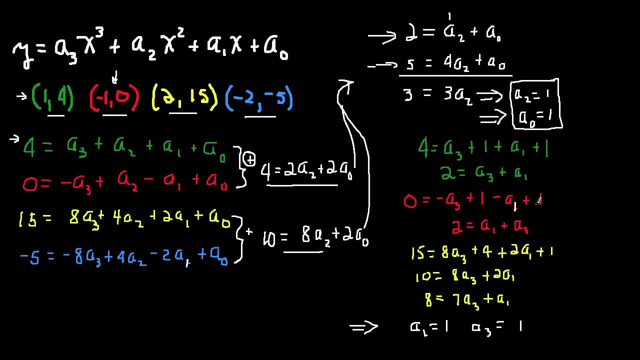 This is a1 plus 1 because a0 is 1.. So this is plugging in a2 equal 1 and a0 equal 1 into the red equation And I get 2 is equal to a1 plus a3.. Well, this is the same equation as this one. 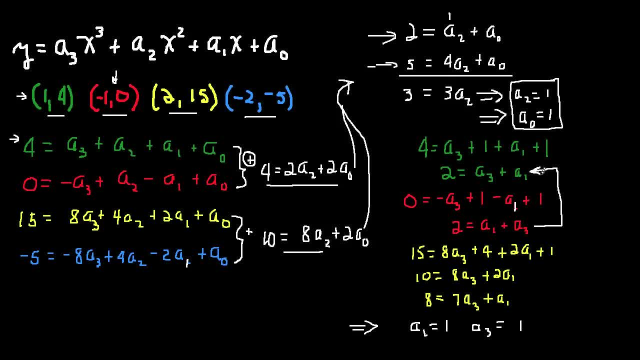 So I can't solve these two because I've only got one equation and two unknowns. Let's try the The yellow equation: I get 15, equal to 8a3 plus 4a2, and a2 is 1, plus 2a1 plus a0, which is 1.. 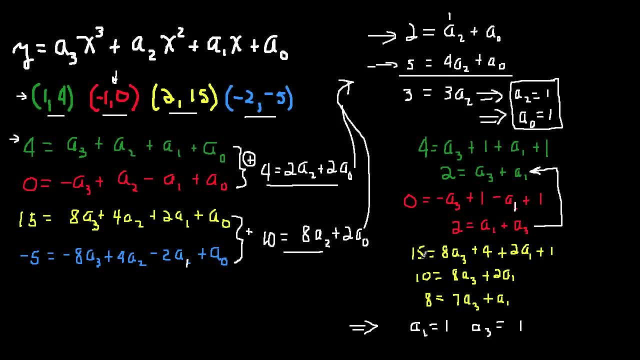 So I get. So I have this: 4 plus 1 on this side And I'm going to subtract that 5 from both sides, That gives me 10 is equal to 8a3 plus 2a1.. That's after I've got rid of these two constants here. 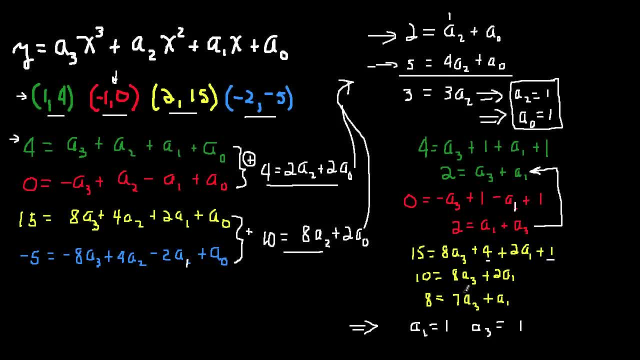 And here that's where the subtracting 5 from both sides I can. So I now have this equation for a3 and a1.. And I have this equation for a3 and a1. So I can subtract this equation here. 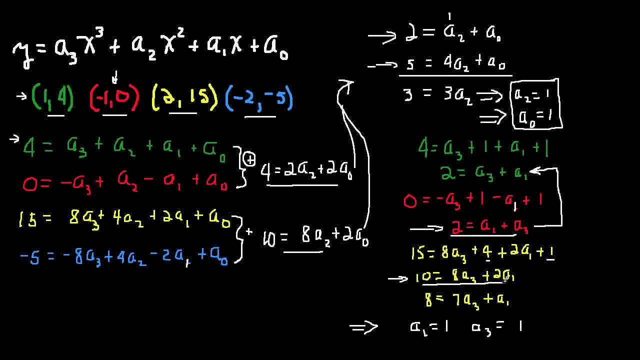 I subtract the red equation from this yellow equation, That gives me 8 is equal to 7a3 plus a1.. So I now have my two equations and two unknowns. I have this equation and I have this equation, which are not the same equation, and I can. 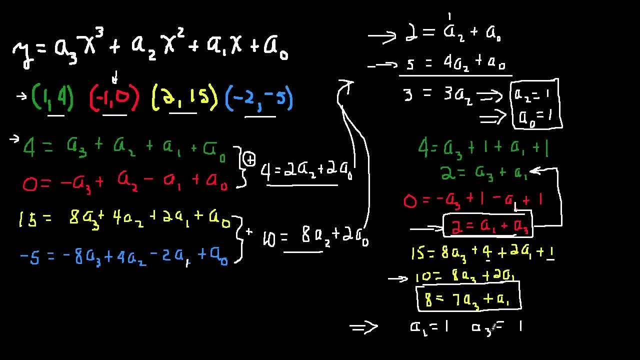 solve those for a1 and a3.. I don't go through the details, but here's the answer: A1 is equal to 1 and a3 is equal to 1.. So it is possible then to solve using four points. We can find four coefficients. 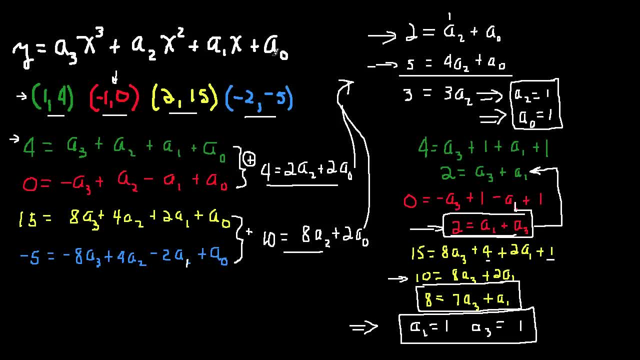 Okay, And This is generally true, If we have a fourth degree polynomial, we need five points. If we have a fifth degree polynomial, we need six points, Because a fifth degree polynomial will have six coefficients, Remember the a0.. So here this is a general rule that, depending on the order of the polynomial we're going. 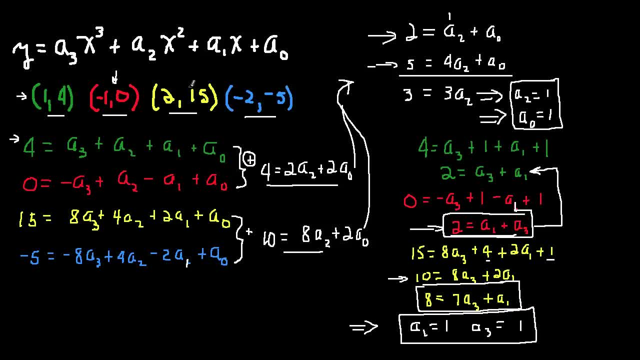 to need that many points, plus one more, To be able to determine the equation of the polynomial, determine the coefficients of the polynomial. Okay, Now let's say here we have our answer. We have: y is equal to x cubed plus x squared, plus x plus 1.. 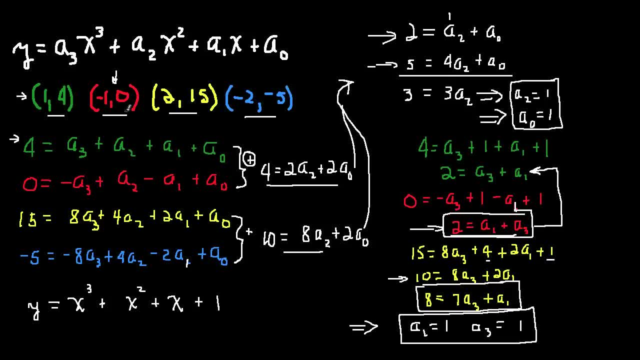 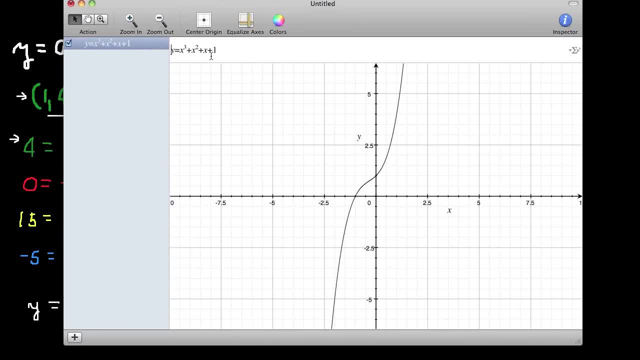 So this is the polynomial that we have that goes through these four equations. Okay, Thank you. Let's see if I plot that out. Here's a plot of that polynomial: X, cubed plus x, squared plus x plus 1.. See, does it go through the four points? 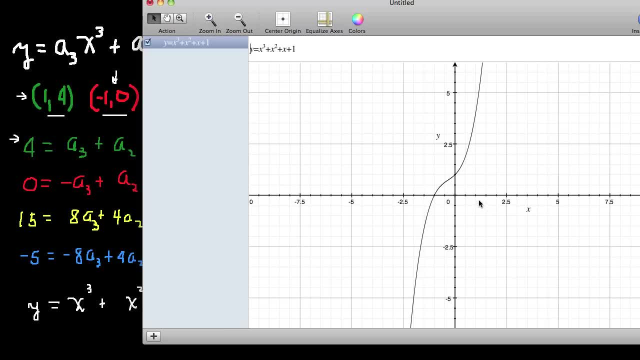 Does it go through the point x equal 1 and y equal 4?? Well, let's see, This is x equal 1, right here, And this would be y equal 4, right here. So it looks like it goes through that point. 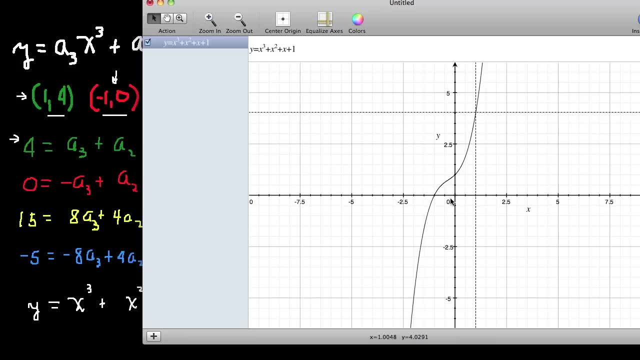 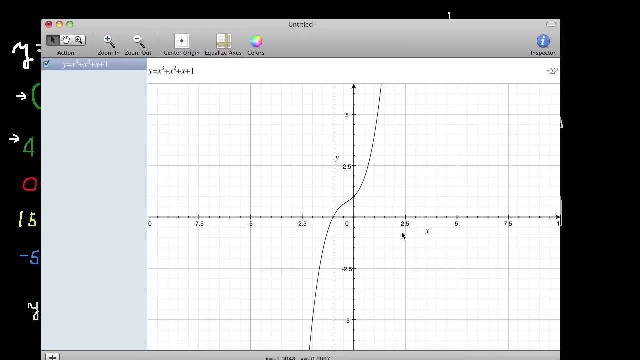 Does it go through the point negative 1, 0? Say, if this is negative 1, then this is 0. So it goes through that point. Does it go through the point 2, 15?? 2 would be here. 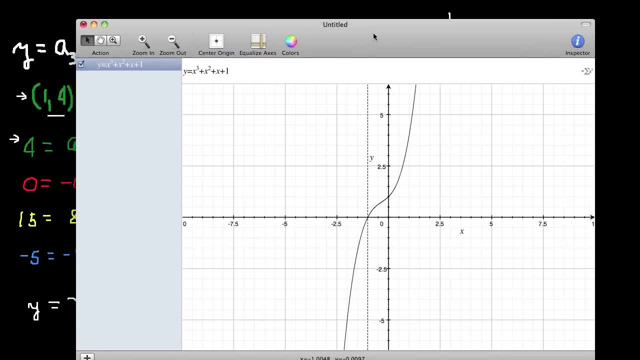 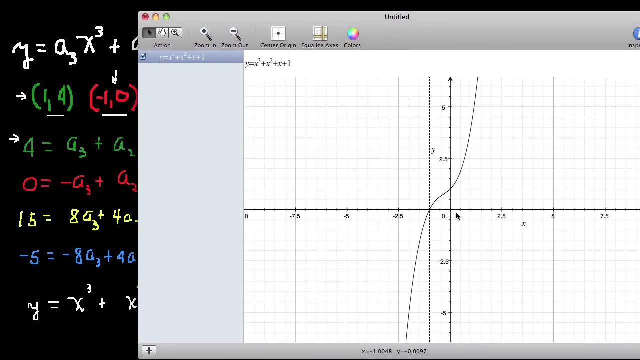 Actually, I can't tell if it goes through 15.. It just looks like it does, though, And does it go through the point negative 2, negative 5?? So I go here to negative 2, which is: this is 0, 0, right here.